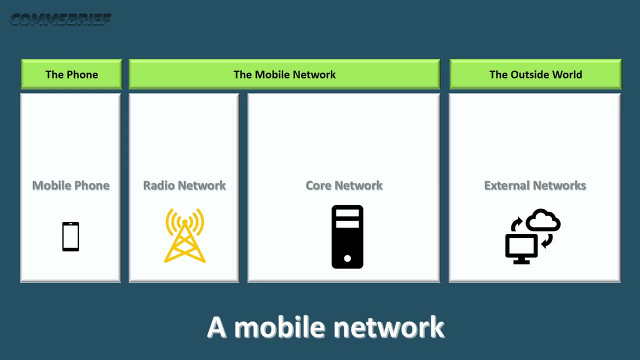 are part of the radio network. The core network is basically the brains of a mobile network. Now, if the core network is the brains of a mobile network- and since I have started this human analogy and of course I'm going to have to continue with that- I think we can say: 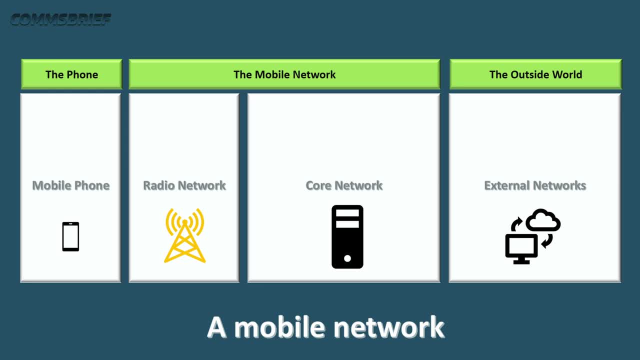 that the radio network is the arms and legs of a mobile network. Why am I saying that? Because it provides the reach, so the network can reach your phone wherever you are. Finally, we have external networks that represent the outside world, so your mobile network. 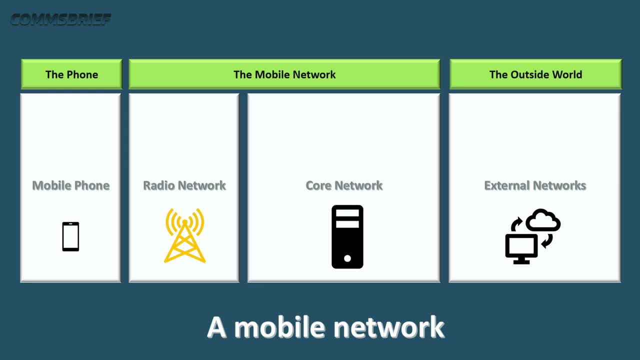 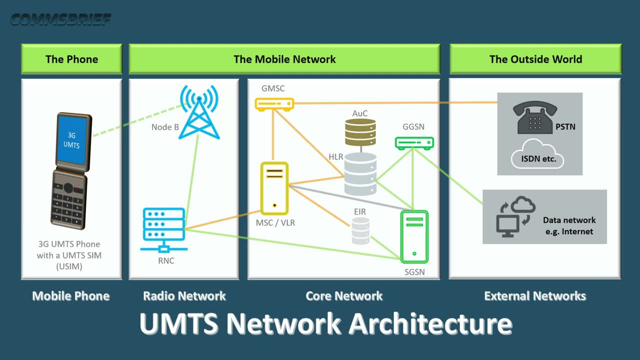 can connect you to telephone networks and the internet. Now let's have a look at the 3G UMTS network architecture. I guess for some of you this might be simplified and for some others it might not be. But don't worry, we will make it even simpler. Let's remove all of these lines. 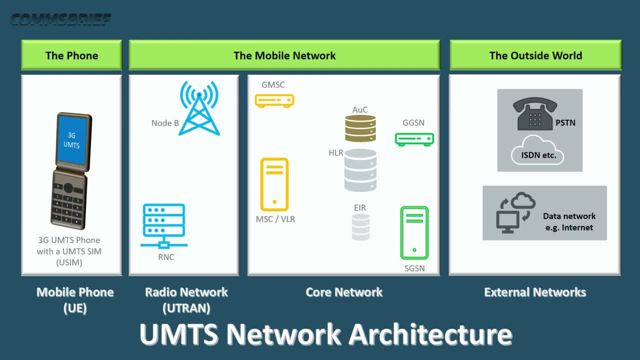 so we just look at the network elements first. Okay, now it looks a bit simpler. Starting from the left, we have a mobile phone, also known as a cell phone. In 3G UMTS networks the mobile phone is called user equipment or UE. 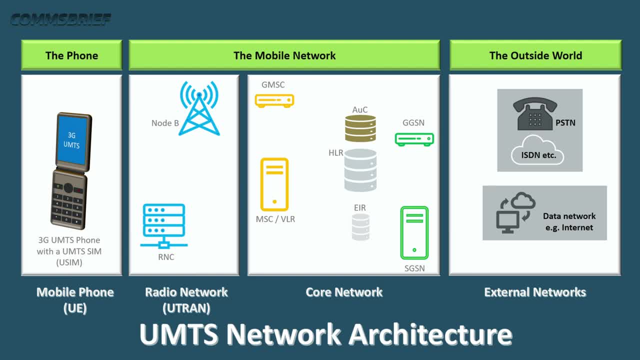 A 3G UMTS phone can take in a UMTS SIM or USIM. Moving now slightly to the right, we have the radio network consisting of a cell tower called NodeB and a radio network controller or RNC. 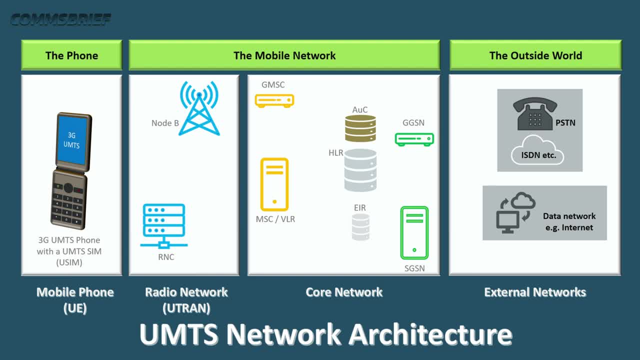 Both these network entities form a 3G UMTS radio network called the UMTS Terrestrial Radio Access Network or UTRON. Quite a mouthful. it is Moving to the right again we have the core network, which has quite a few entities. 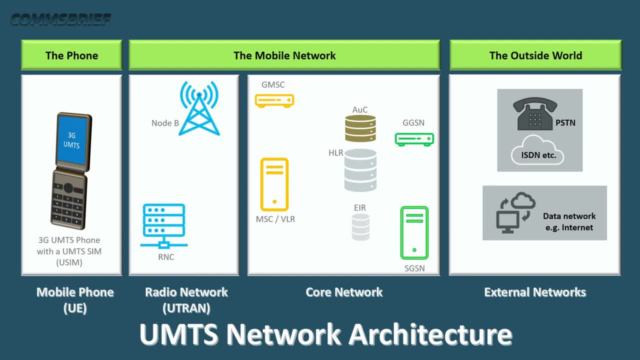 In the middle we have all the databases like the Authentication Center, AUC, Home Location Register, HLR, and Equipment Identity Register, EIR. You may have noticed that we also have MSC and SGSN in the 3G UMTS core network. 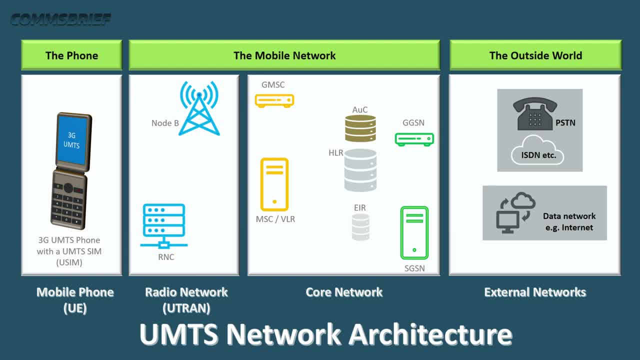 just like in the GSM network with GPRS enhancement. In this diagram I have kept the MSC and GPRS enhancement. In this diagram I have kept the MSC and GPRS enhancement GMSC in orange color and the SGSN serving GPRS support node. 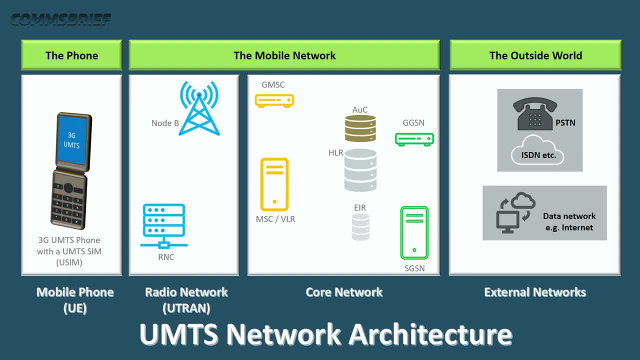 and GGSN Gateway GPRS support node in green. So the orange color here represents the circuit switch part and the green color represents the packet switch part. But what exactly is circuit switch and packet switch? I'm sure you're wondering. 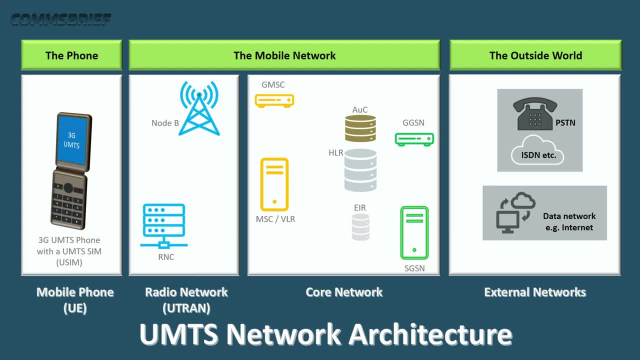 Circuit switch is a conventional technology where dedicated circuits are used for communication. It is not very efficient because the communication link is established for the entire duration of the call, even when someone is not talking or doing anything. Packet switch, on the other hand, is very efficient. 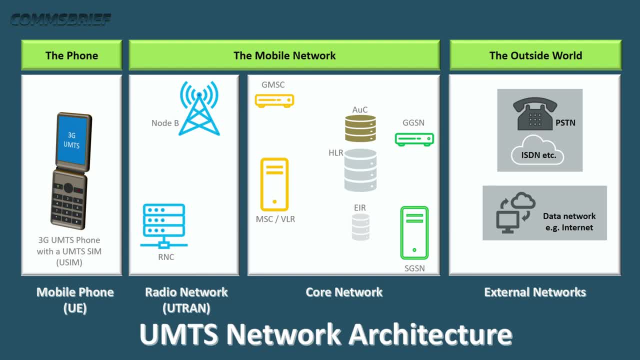 and that's why it is used for mobile internet or mobile data. So the orange boxes here are for the circuit switch, voice calls and text messages, and the green boxes here are for mobile internet. The 3G UMTS network, just like GSM networks, uses circuit switch for voice calls and text messages. 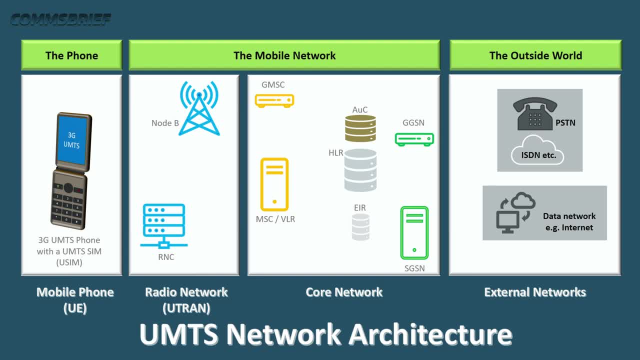 SMS. SMS and text messages are the same thing, so SMS stands for short message service. Finally, in this diagram we have the last part here, which is the outside world, consisting of many, many networks, including PSTN and ISTN, etc. for circuit switch. 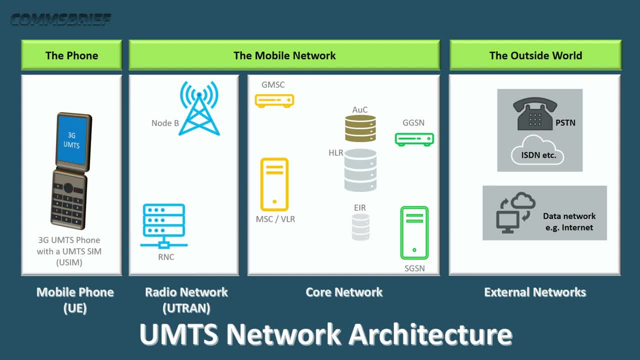 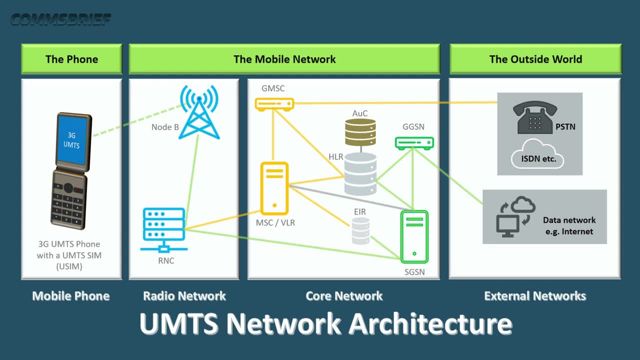 and data networks like the internet for packet switch. Now let's bring back all the lines so we can see which network can take place and which entity is connected to what. Now, with all of these lines, you can see how these network elements are connected to each other. 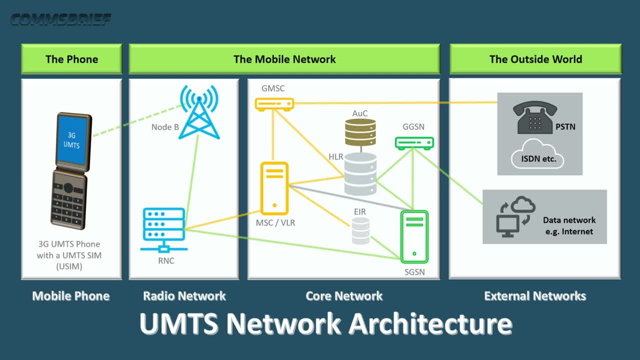 The 3G UMTS phone talks to the node B for any communication. Node B is connected to the RNC or radio network controller. RNC is the boss of node Bs. One RNC can control many, many node Bs. The equivalent of RNC in GSM networks is the BSC or base station controller. 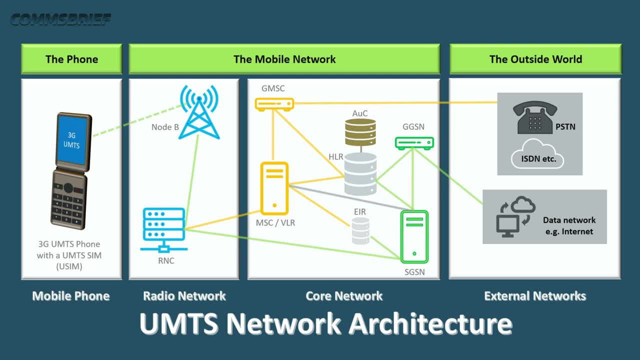 The RNC connects to the MSC for circuit switch services like voice calls and text messages, and it also connects to SGSN for mobile internet services. The MSC is connected to the outside world, like PSTN and ISTN, via Gateway MSC or GMSC. 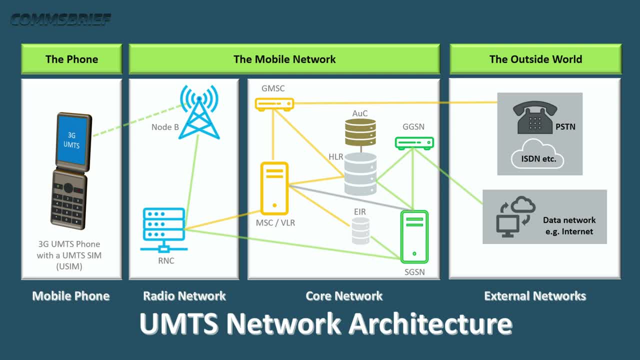 The SGSN is connected to the outside world like the internet via Gateway, GPR support node or GGSN. Then in the middle we have all of these databases like Authentication Center, AUC, HLR and EIR and VLR, of course. 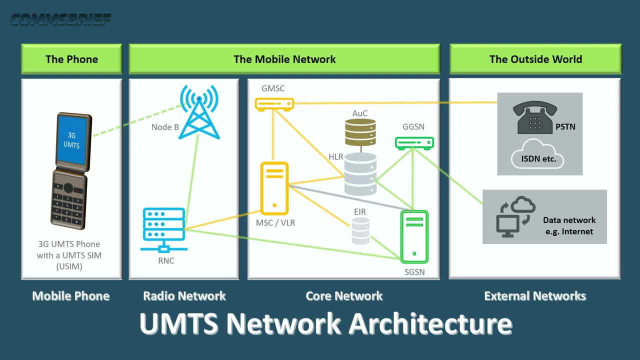 Authentication Center, AUC, validates the SIM card and uses ciphering so the phone can securely connect to the mobile network. HLR is the Home Location Register, which contains information about your home location, as the name suggests. of course, right, it says that in the name and the services you're entitled to use. 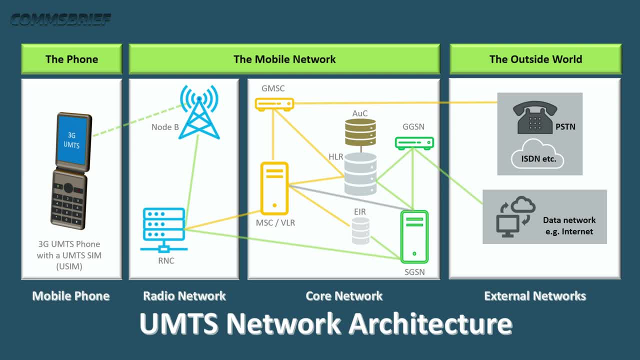 HLR is a centralized database. Then we have VLR or Visitor Location Register. VLR is a decentralized or distributed database that keeps the HLR updated on the location and service status of users. Finally, EIR is the Equipment Identity Register. 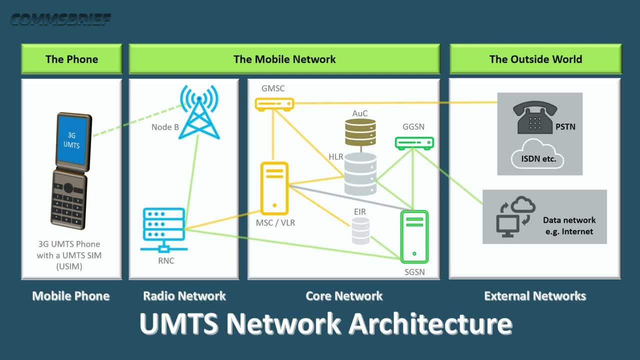 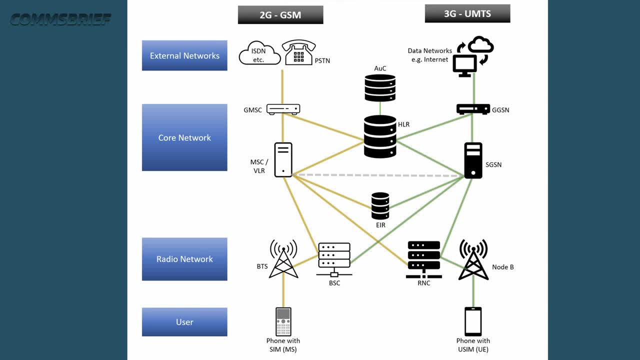 and it is a database where all the IMEI numbers that are registered on the network are kept. And now I just wanted to show you this combined GSM and UMTS network architecture And it is very important because UMTS networks were not launched to replace 2G GSM networks quickly. 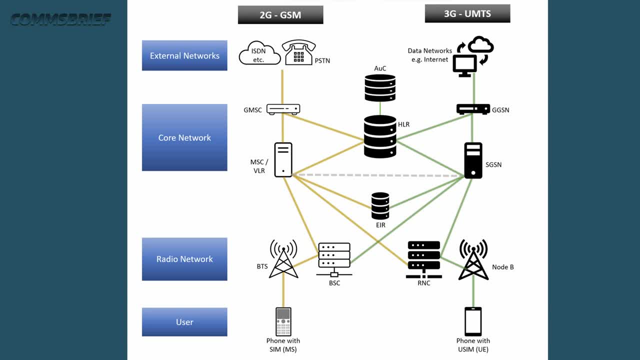 but they were expected to coexist with them for a very long time. And what is a very long time? Well, GSM networks still exist today, even in 2023, three decades after the first launch of GSM in 1992.. So that, I'm sure, is a long time. 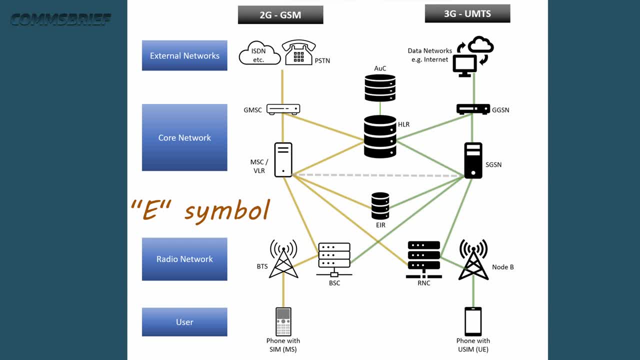 Every time you see an e-symbol on your phone, you're connected to the GSM network. So the best way to look at 3G UMTS network architecture is to see how it fits with the earlier generation GSM and the later generation 4G LTE. 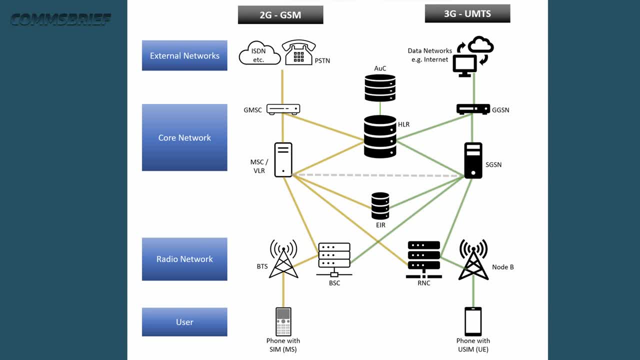 I'll cover the 4G LTE part of the architecture in a separate video. Now, as you can see in this diagram, there is a lot of symmetry here. The mobile phone is called Mobile Station, or MS in GSM, And user equipment or UE in UMTS. 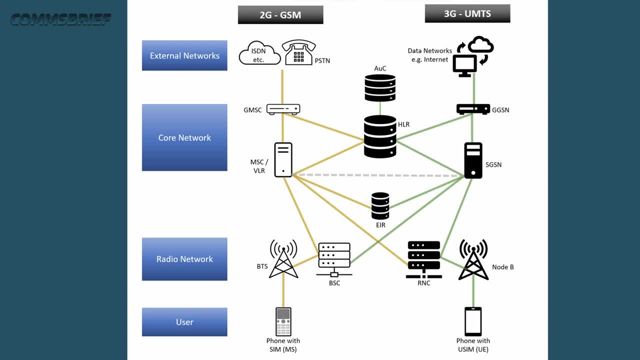 The base station is called BTS in GSM and NodeB in UMTS. The base station controller is called BSC in GSM and RNC in UMTS. The MSC and SGSN are used in the same way in both GSM and UMTS.